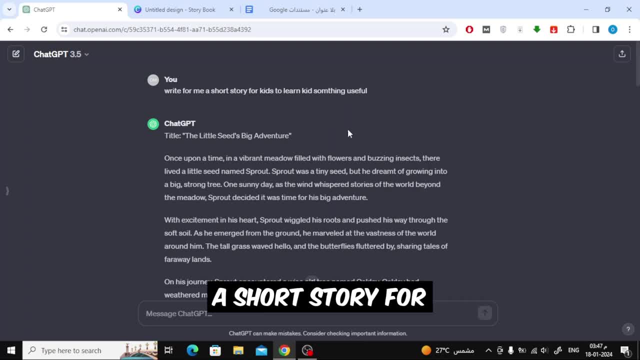 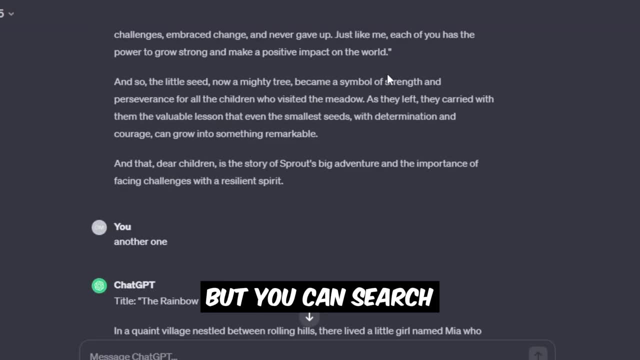 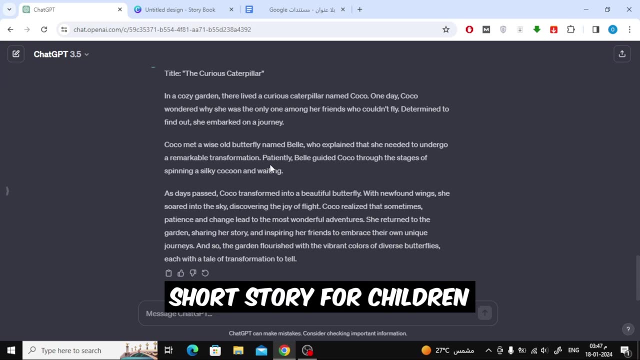 and artificial intelligence text generator. Write for me a short story for kids to learn something useful. Here I use the easiest prompt you can use to generate a story for children, But you can search more on the internet for more professional prompts. NowChatGPT has created a useful short story for children. It is the story of a caterpillar that 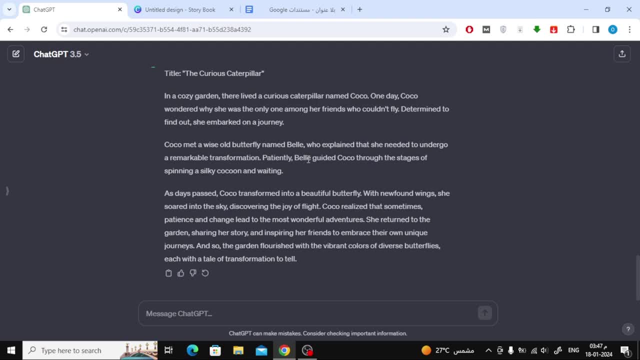 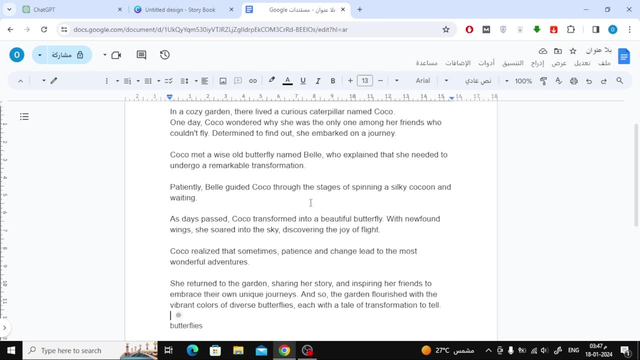 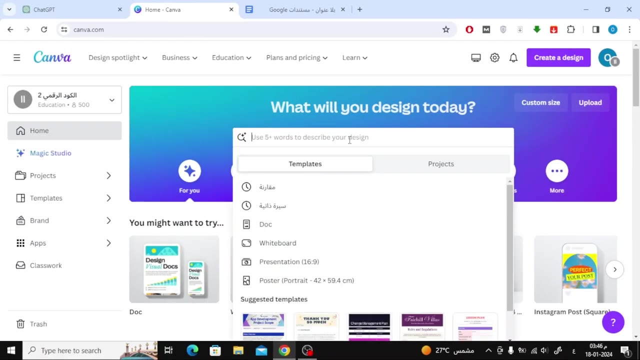 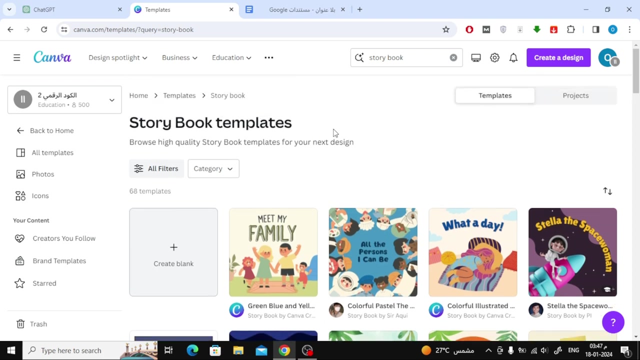 feels sad and wants to turn into a butterfly, like its friends. I will now copy the story and paste it into Google Docs for us to use later. Now go to the Canva website and type in the search book story. Now click on the create blank option so that we open a page that is the appropriate size for the 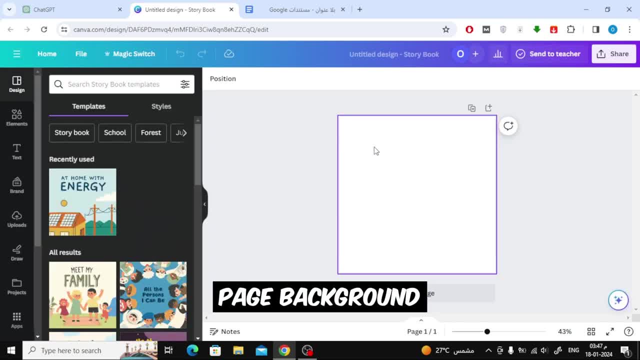 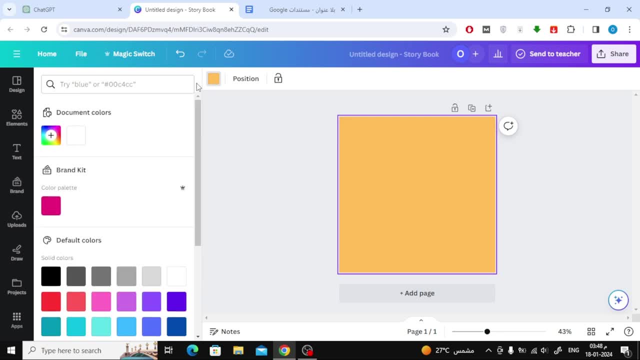 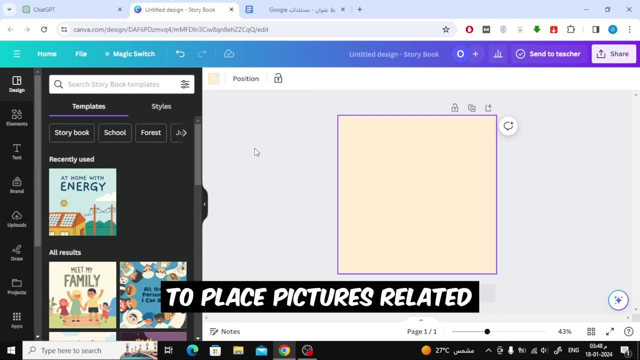 story. The next step is to change the page background to a different color. Here I have chosen this color. Now we want to add a frame to place pictures related to our story inside it. Go to the elements section and type in the story. 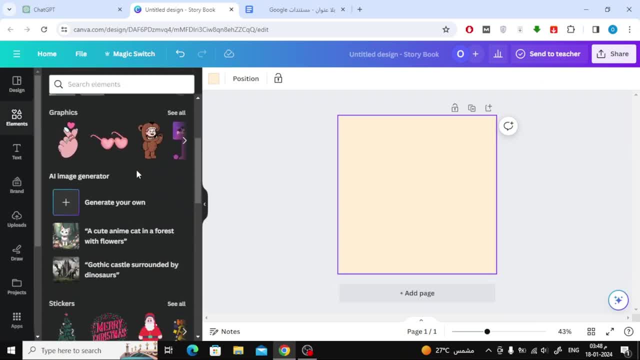 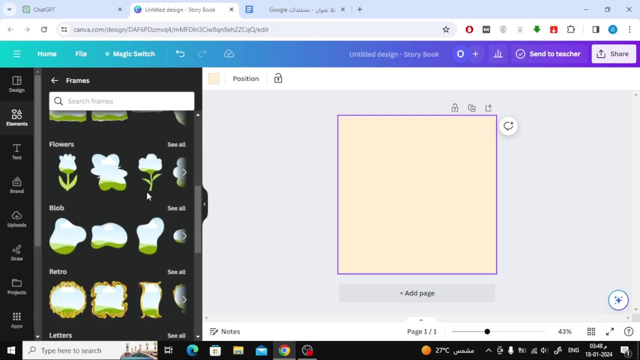 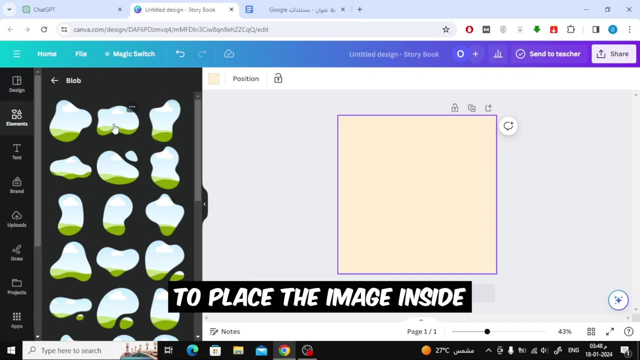 Then open the frame section. After that open the blob section. I will use these shapes in my book to place the image inside. Now browse these many shapes, then add the one you like. Next, add the first section of a story as text on the first page. 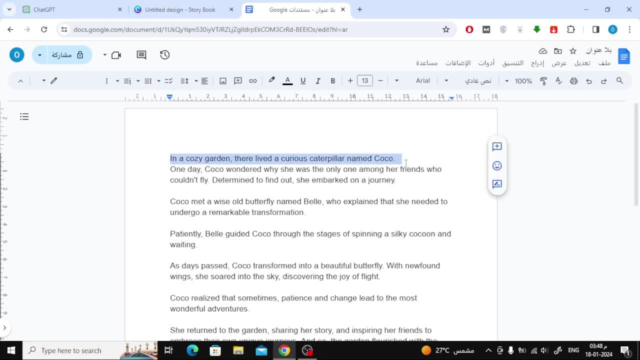 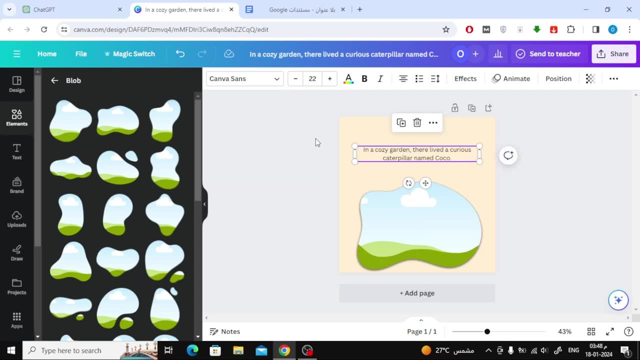 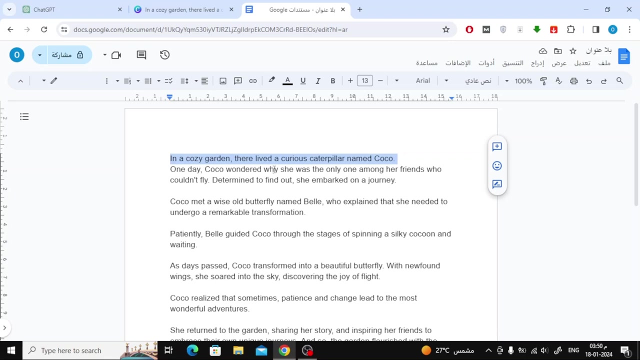 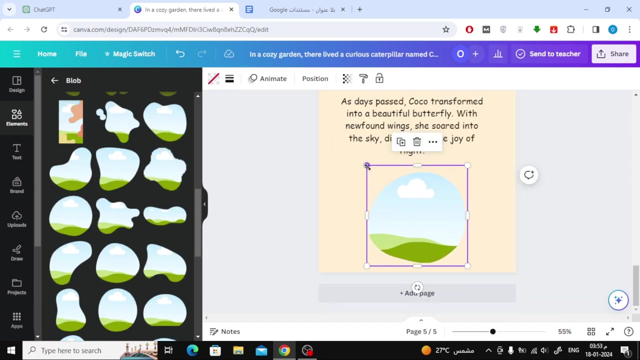 After that, change the font type of the text to Comic Sans. In this way, I complete the creation of the rest of the pages of the story. Add story lines on each page in an appropriate manner. Use the logo to add to this text. 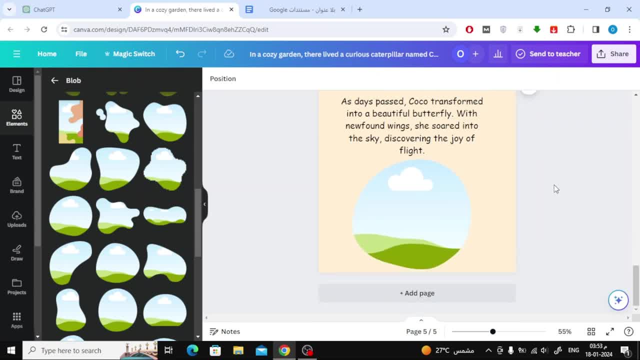 You can actually add a title to the title of the text. if you want to Click on add to title, Then click on the title to add to your text. Now we are going to add an option to our story Here. we are going to write a text in the title of our story. 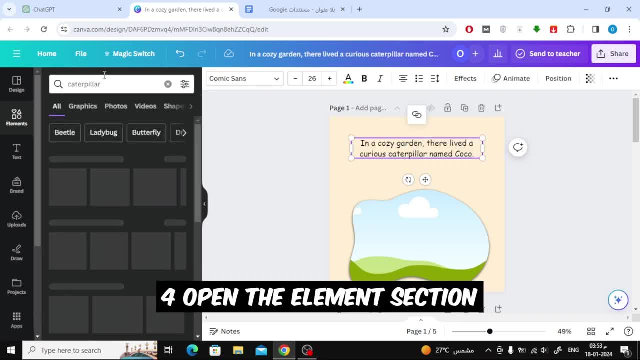 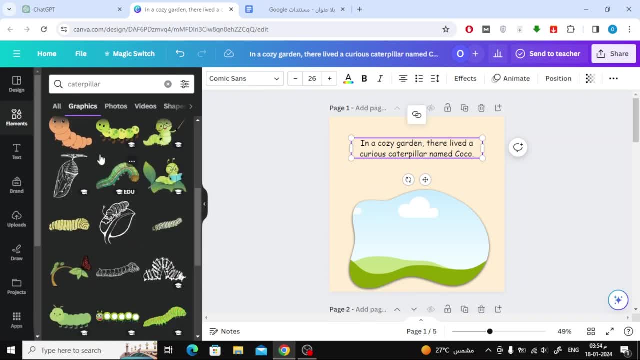 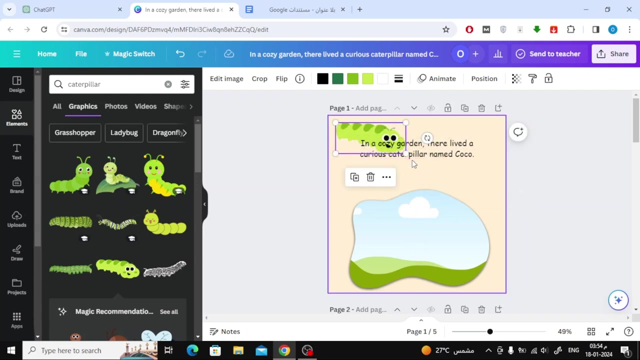 The next step is to add decoration to the pages. Open the elements section, then type caterpillar in the search box. We will add one of these cute pictures from the graphics section to the front page. After that, open the transparency and reduce the value to 40.. 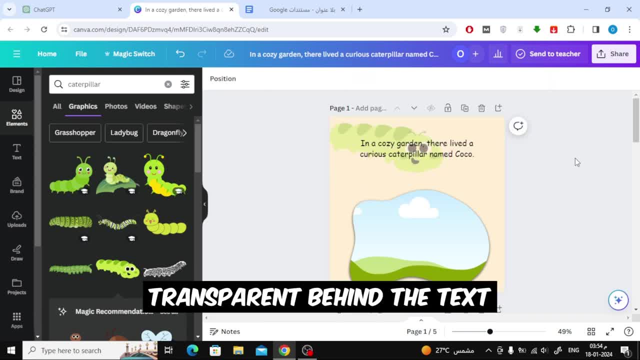 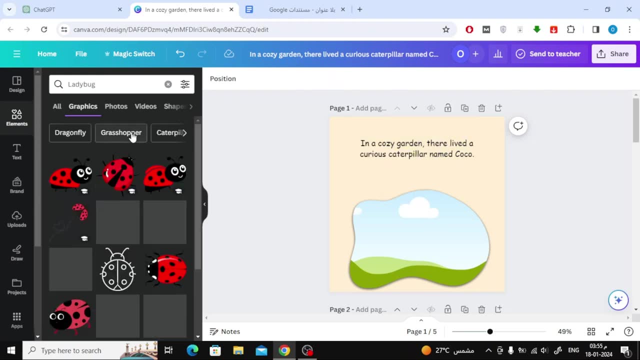 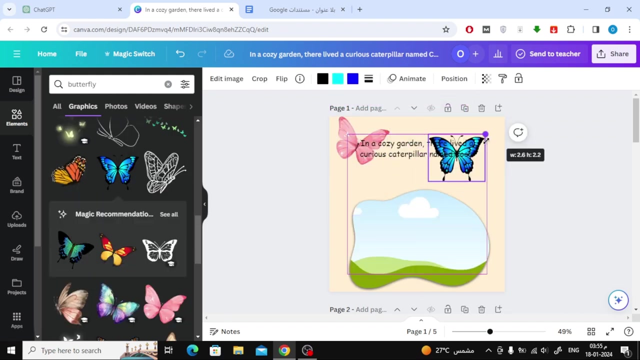 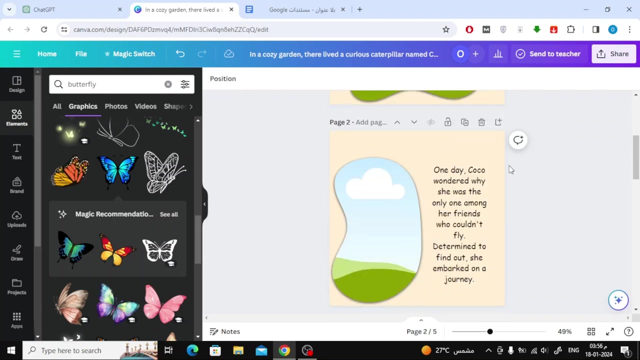 We want to make the image of this caterpillar transparent behind the text, to give aesthetics to the page In this way. continue adding interesting shapes and images to the rest of the pages, then make them semi-transparent. If you liked this video, subscribe to our channel and click the bell to receive notifications of our latest videos. 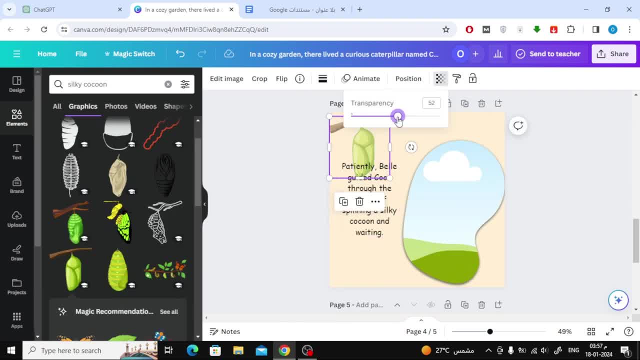 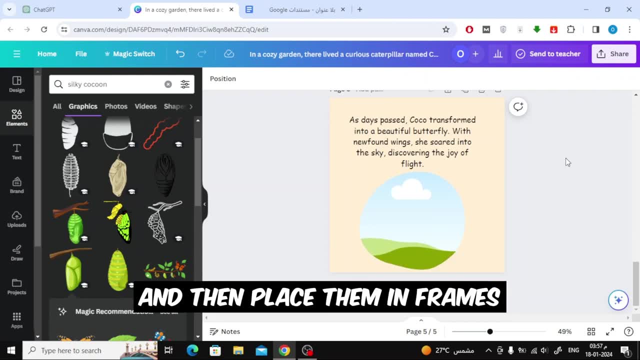 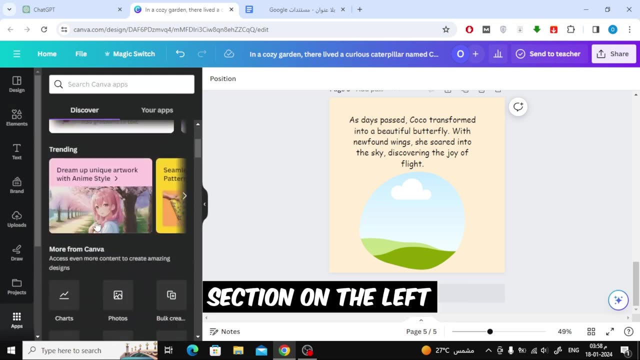 Thank you. The next step is to create images that relate to our story and then place them in frames. We will now use Canva's free image generator. Open the applications section on the left, Then scroll down and click on magic media. Here I will write: garden. 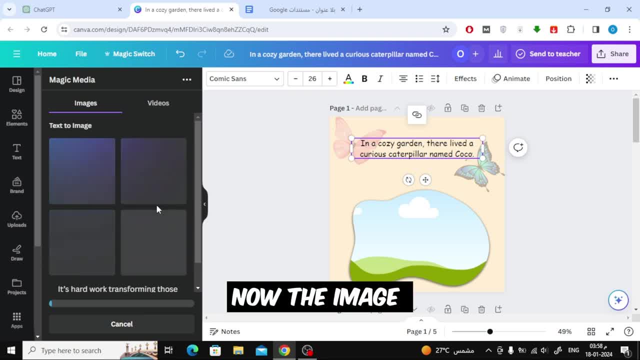 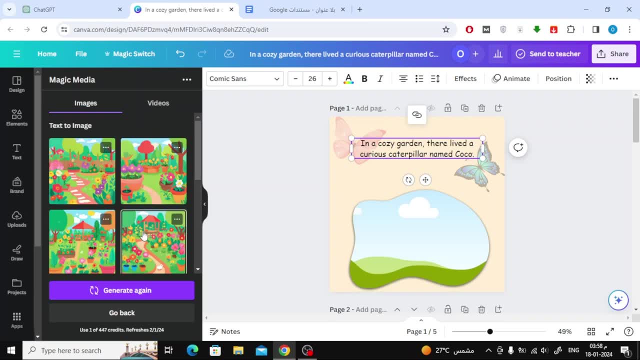 Then I will choose the playful option from the styles. Now the image generator will create a garden image that we will place on the first page of our story. I will now add a picture of the caterpillar. As you can see, I am now adding one of the pictures to the frame. 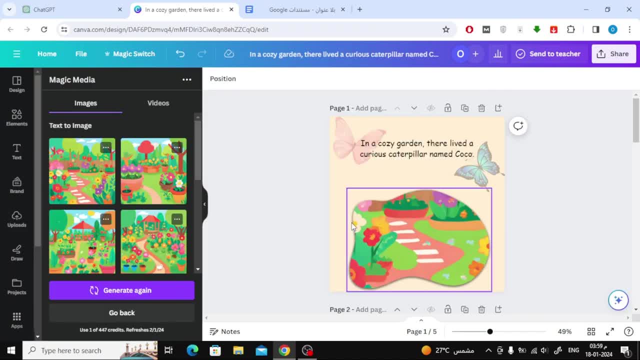 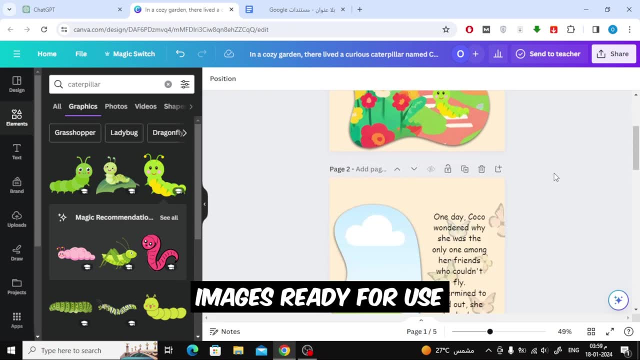 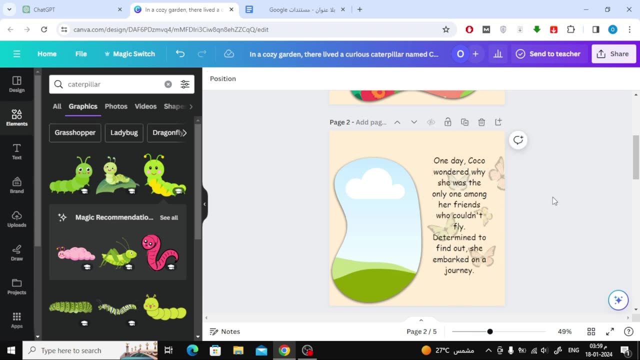 I will then add a picture of the caterpillar. In the elements section there are a lot of images ready for use in case the image generator is not working well. On the next page, I will create an image of butterflies flying in the garden. Now I will add a picture of the caterpillar flying. 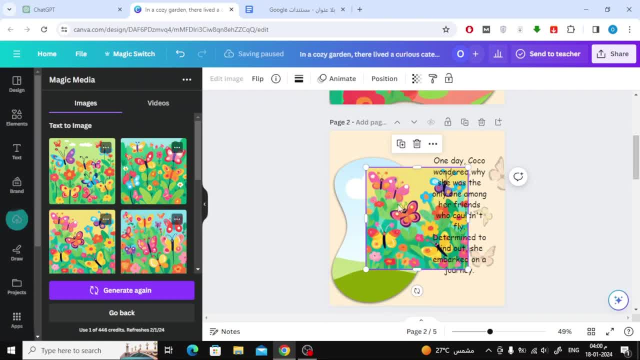 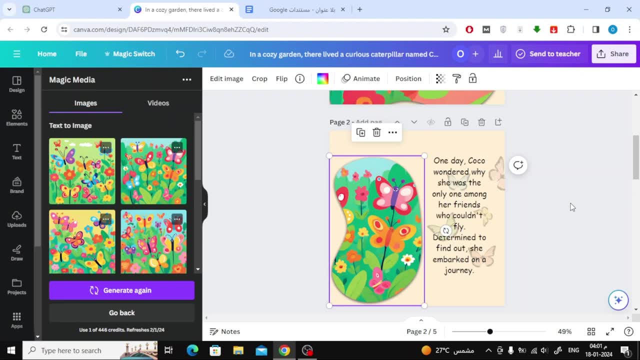 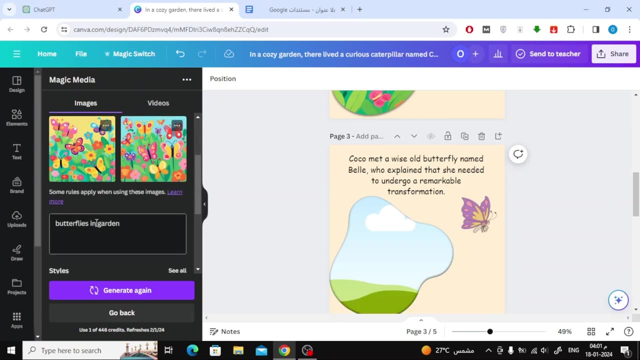 Then I will add a picture of the butterfly flying in the garden. Now I will add a picture of the butterfly flying in the garden. Next, on the next page, I will create an image of a wise butterfly and place the caterpillar next to it.